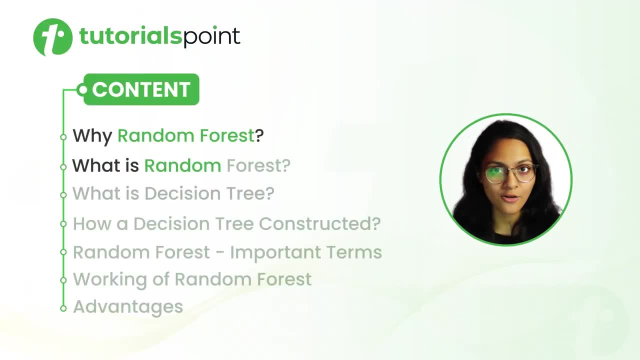 We are going to look at why random forest, What is random forest? What is decision tree, How a decision tree constructed, What are the important terms of random forest, What is the working of random forest And what are the advantages of random forest. 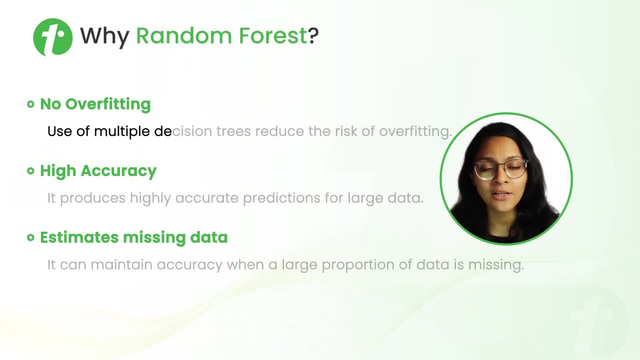 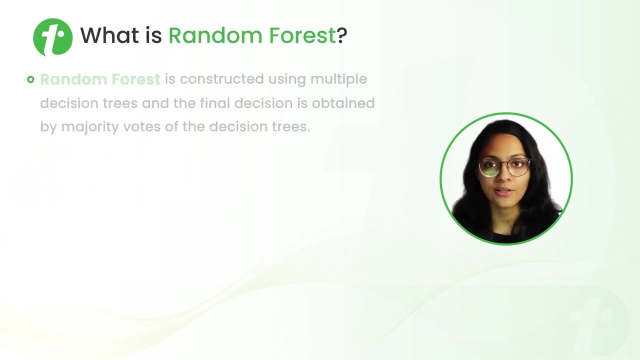 First is why random forest- Random forest- uses multiple decision trees, so it will reduce the risk of overfitting. It produces highly accurate predictions for a large data And it can also maintain the accuracy when a big portion of the data is missing. Now, what is random forest? 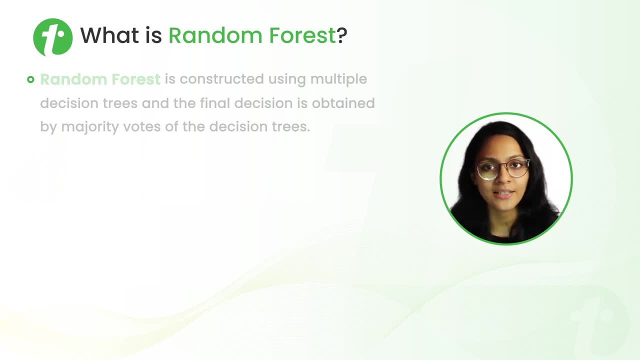 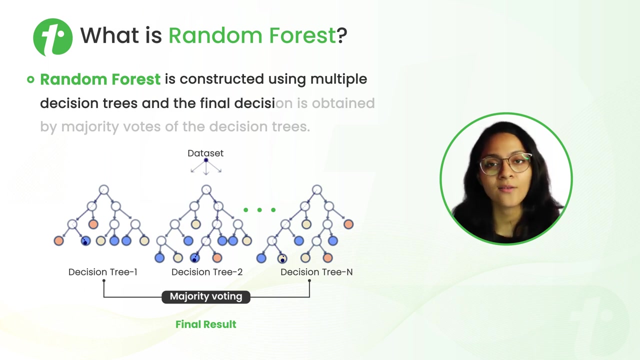 Before that, can you tell me what is forest? Obviously, the group of random trees is called forest Correct. Similarly, random forest is constructed using multiple decision trees. And how does we take the final decision? in random forest algorithm, The final decision is obtained by the majority votes of the decision trees. 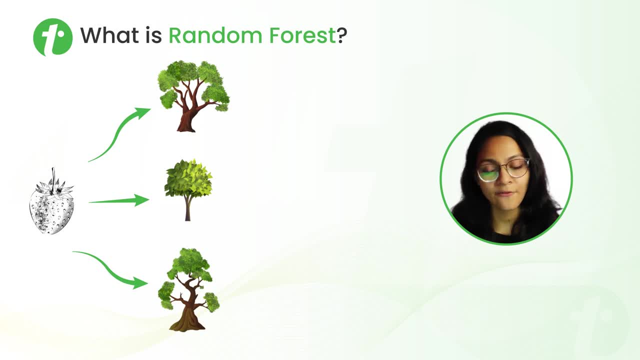 Let's understand this with an example. Let's say we have these random decision trees And we provided some unknown root to these decision trees. Now the first decision tree is predicting that it's a strawberry. Second decision tree is predicting it's an orange. 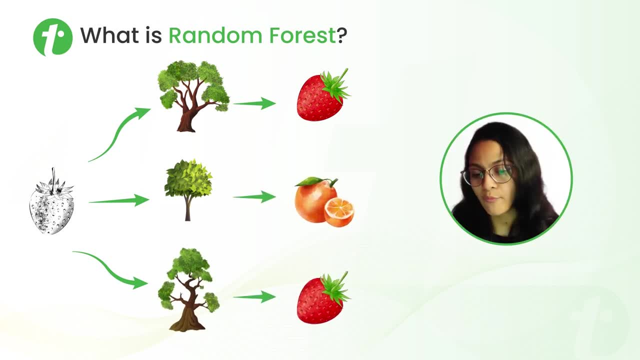 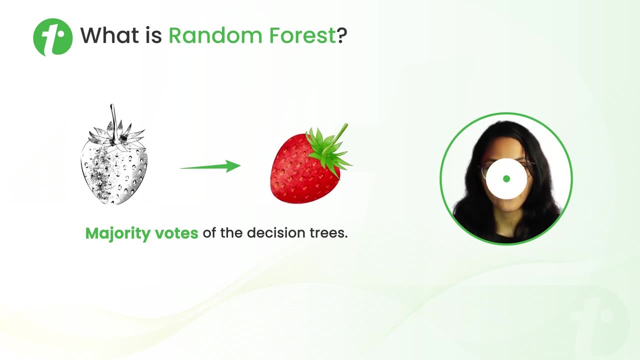 And third decision tree is predicting it is a strawberry, So we have majority votes for strawberry, So our final decision will be the given unknown root is a strawberry. Now, before understanding the random forest, it's important to understand the decision tree. 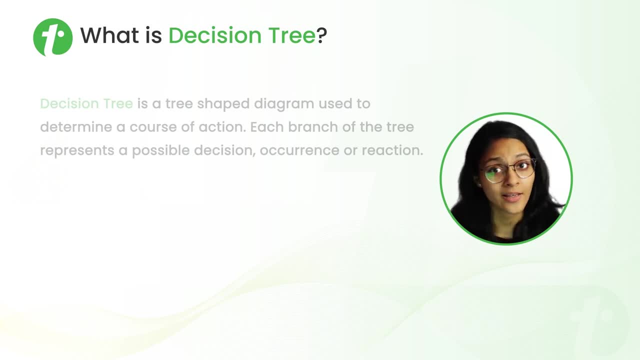 Because the building blocks of the random forest is a decision tree. So what is decision tree? Decision tree is a tree-shaped diagram which we use to determine the course of actions, And each branch of the tree is called subtree, Which represents a possible decision or occurrence. 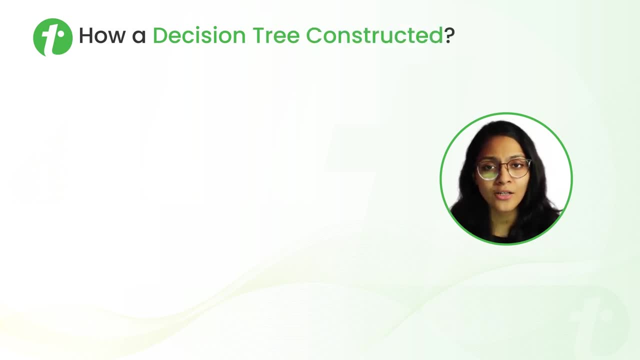 How are decisions reconstructed? It's quite similar to our decisions that we take in our day-to-day life, So let's understand this. with this example, We have to predict the vegetables in this curve. So at the first stage, I am determining whether the color of the vegetable is red or not. 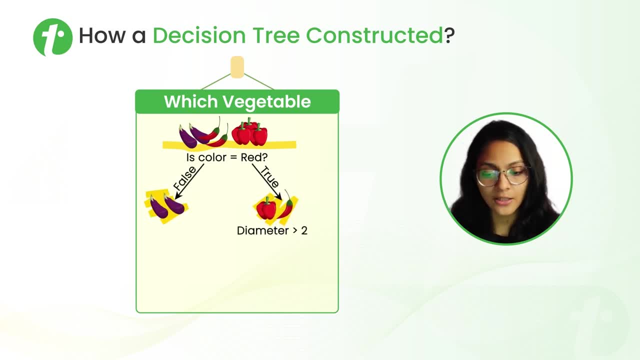 If not, then it is abringent. And if the color of the vegetable is red, then what is the diameter of the vegetable? If the diameter is red, then it is abringent. If the diameter is greater than 2, then it is a red capsicum. 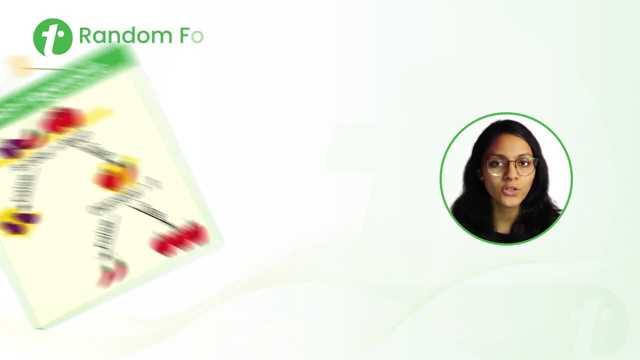 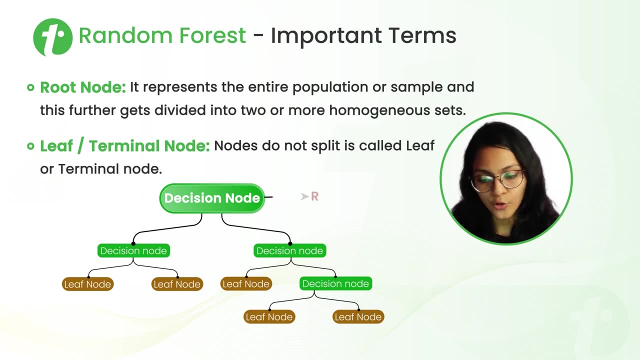 And if it is less than 2, then it is a red chalet. Now let's see what are the important terms of random forest. These are the terms that are also important for decision tree. First is root node. The first node of the decision tree that represents the entire population of the data set is called the root node. 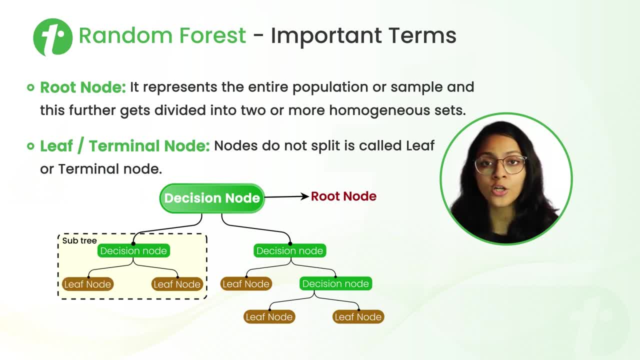 Leaf nodes or the terminal nodes are the nodes that do not split further And also leaf nodes carries the final classification or decision For splitting the decision tree. there are many methods like Gini entropy, And we have discussed the entropy information gain, Gini index in one of our previous videos. that is decision tree. 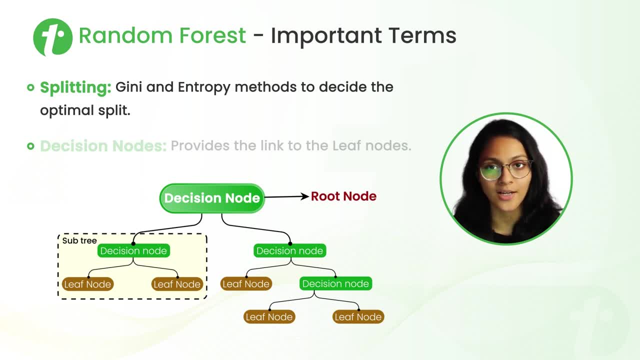 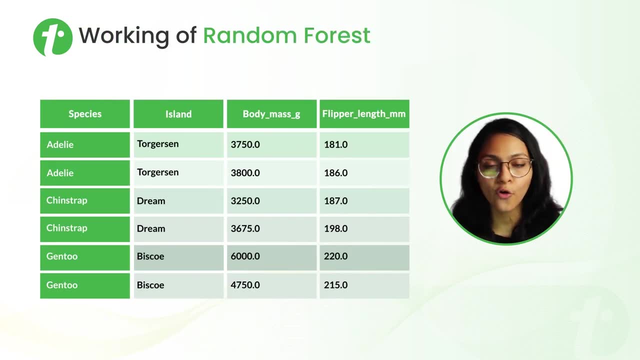 And I suggest you all to watch that video for more understanding. Next is decision node. Decision node provides a link to the leaf nodes. Now let's understand the working of the random forest with an example. This is data set, and in this we have to determine the species of the cute penguins based on some certain features. 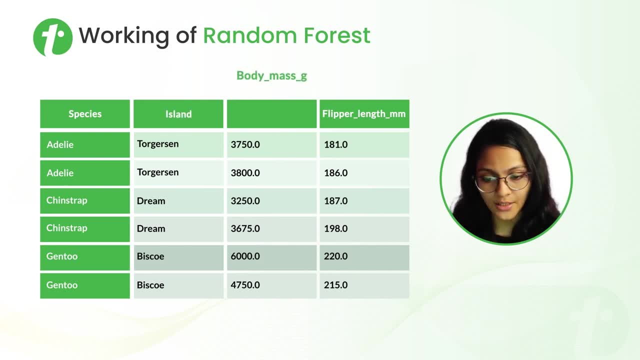 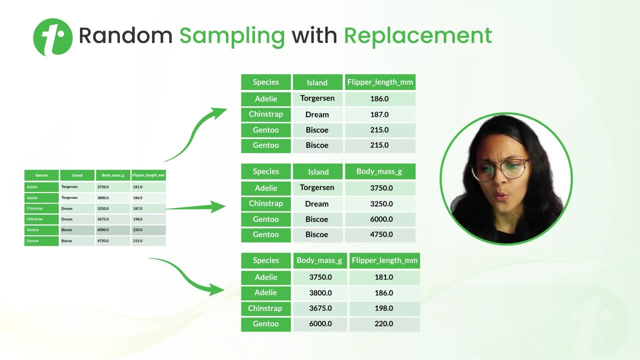 And in this case the features are: island body mass in gram. slipper length in mm. Now we have to do the random sampling with replacement for the given data set. What does this random sampling mean and what does this replacement mean? 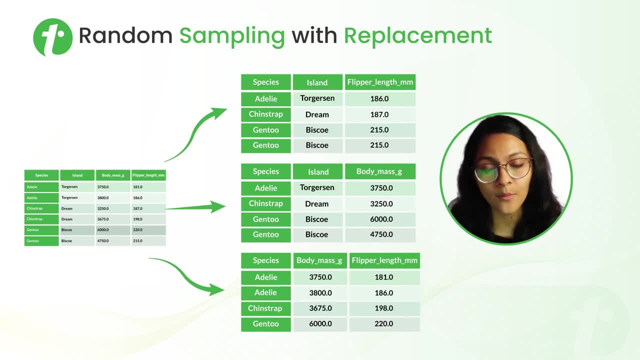 Random sampling means that we have to select some random rows and random features and make some random samples. So here we are, selecting random rows and random features and making these three random samples. What does this replacement mean? now, Replacement we can understand from the first random sample. 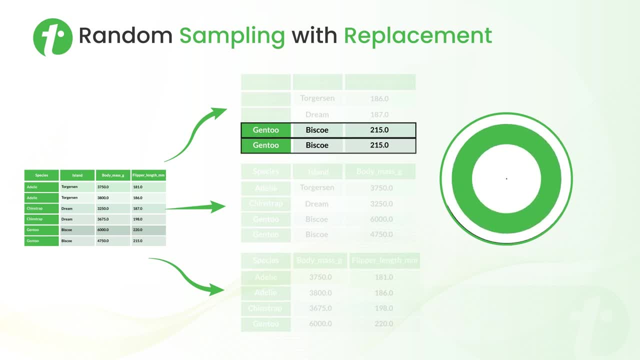 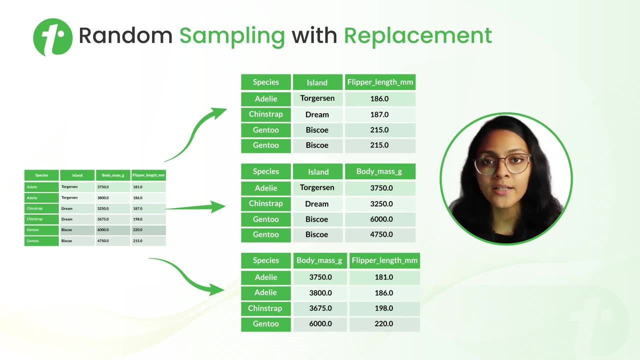 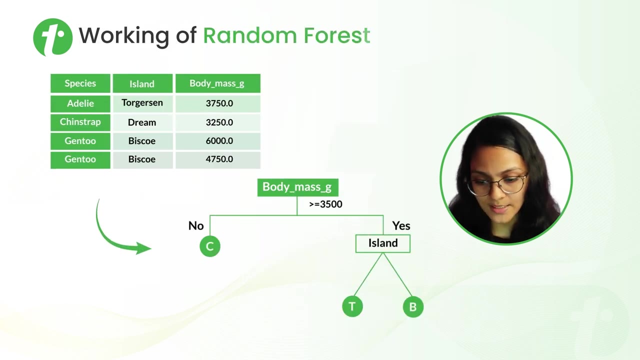 Here this row is repeating. That means some rows are repeating and maybe some rows are not included. So that's what replacement means. Now, after random sampling with replacement, we have to make the decision trees for every random sample. So for first random sample, this is the decision tree. 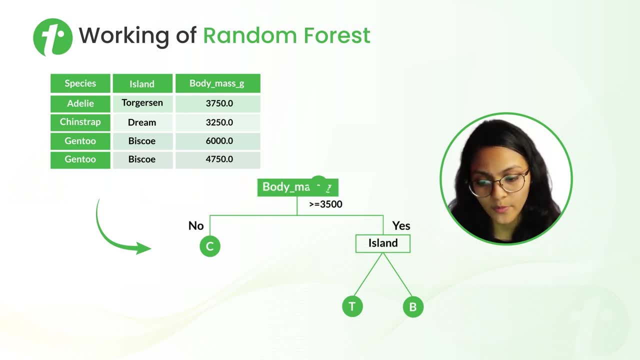 In this, at the first stage, we are determining body mass of the penguin, If it is greater than 3500 or not. If not, then it's a chin strip. If the island is Torgensen, then the species is Adélie. 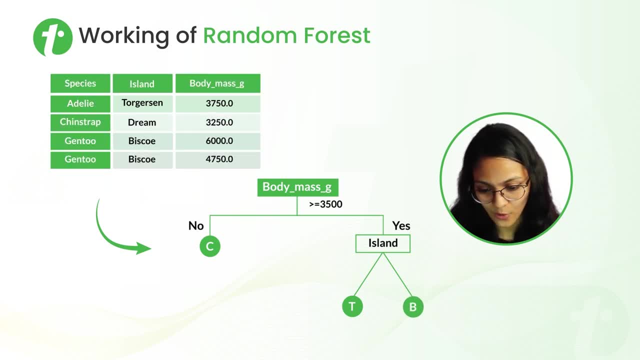 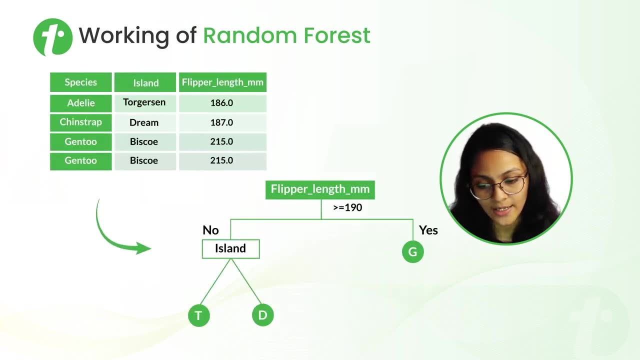 And if the island is Bisco, then obviously the penguin is Gento. This is the decision tree for second random sample And here, at the first stage, we are determining the slipper length of the penguin If it is greater than 190 or more. 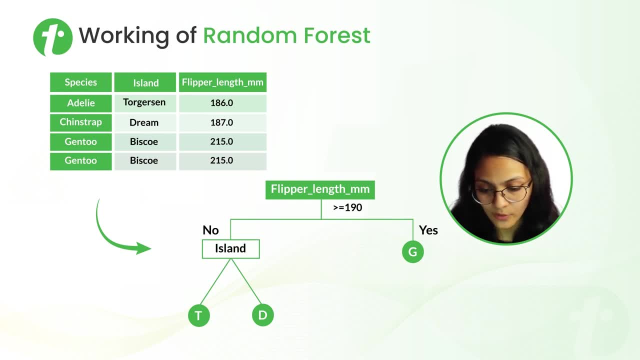 If not, then what is the island of the penguin? Again, if it is Torgensen, then it is an Adélie species, And if it is green, then it's a chin strip species. And if the slipper length is greater than 190, then the species is Gento. 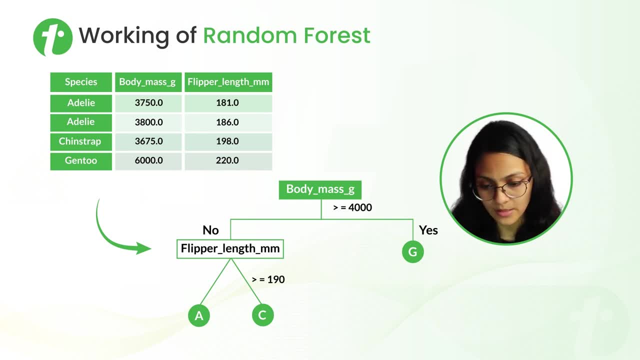 Similarly, we draw this decision tree for the third random sample. Here, at the first stage, we are determining the body mass of the penguin If it is greater than or equals to 4000.. If it is, then it's a Gento species. 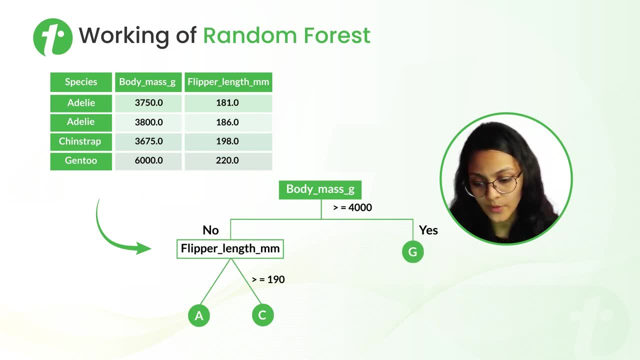 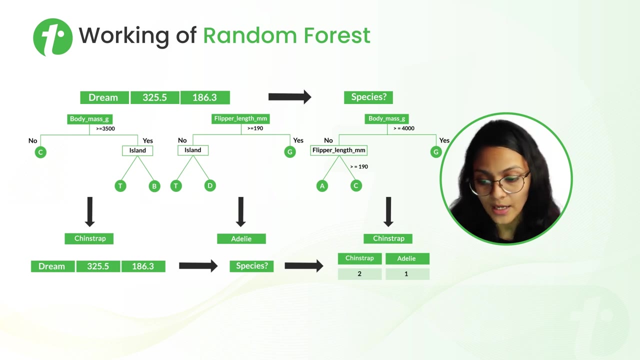 If no, then what is the slipper length of the penguin? If the slipper length is greater than or equals to 190, then it's a chin strip, And if not, then it's an Adélie. Now we have this new input data and we have to determine the species of the penguin. 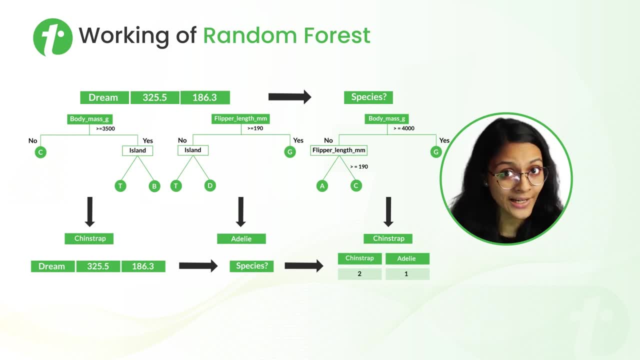 So we give this input to our model that has those three decision trees. So first decision tree is predicting that its species is chin strip. So first decision tree is predicting that its species is chin strip. Second decision tree is predicting that its species is an Adélie. 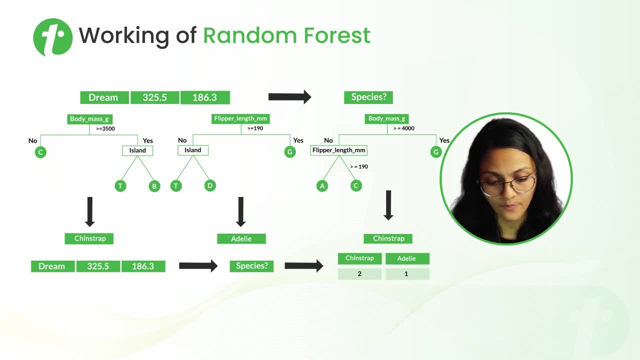 and the third one is also predicting that it's a chin strip. So we have two votes for chin strip and one vote for Adélie. That means the final decision of our random forest model will be that it's a chin strip. Now what are the advantages of random forest? 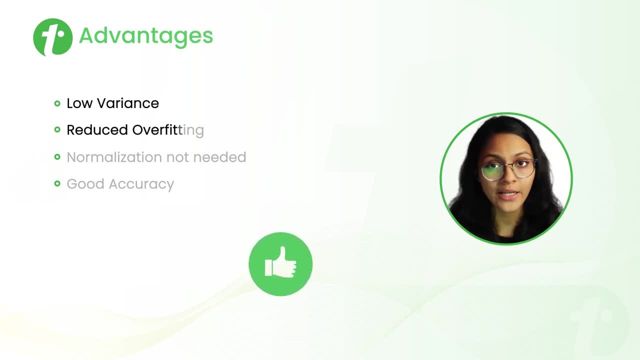 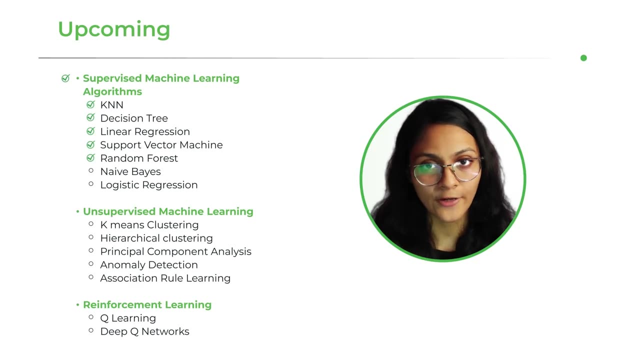 It has low variance. It reduces the overfitting. It reduces the overfitting. Normalisation is not needed in random forests and it has ground and it has good accuracy. so that was it for this video. we have already discussed the supervised 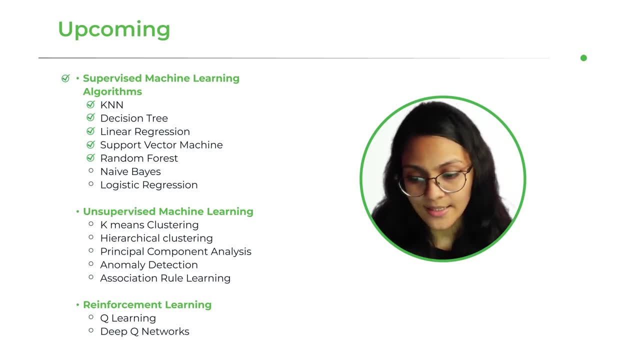 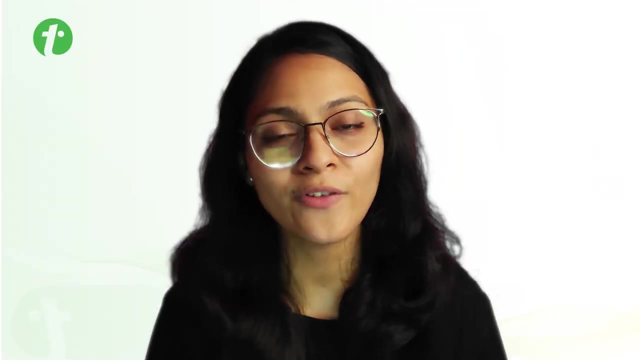 machine learning algorithm, canon algorithm, decision tree, linear regression support vector machine and random forest in this video. in the next video we are going to discuss about knife base and rest- all the machine learning algorithms in further videos. so stay tuned with tutorials point. thanks for watching and have a nice day.